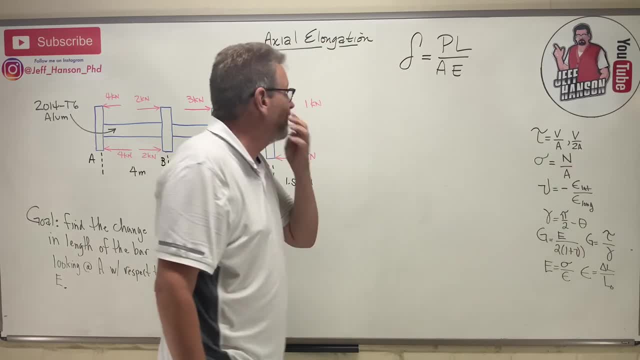 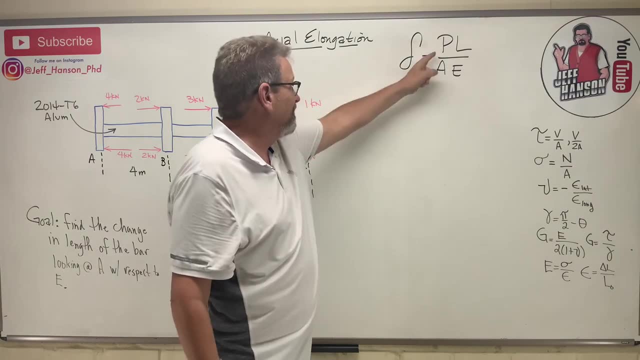 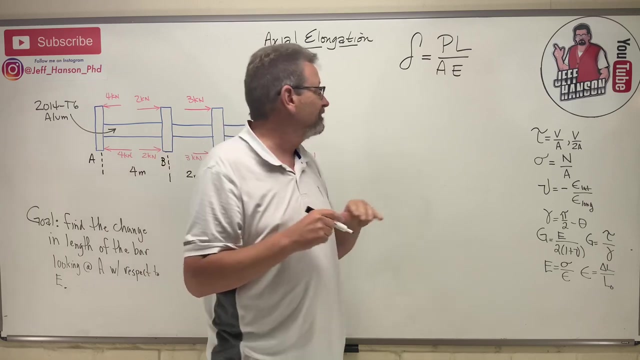 we have P over a, I have n over a written right, but P over a is simply the force, the axial force that's making the beam either longer or shorter. so think of P is standing for push or pull right. so it's either pushing on it or pulling on it, okay L. 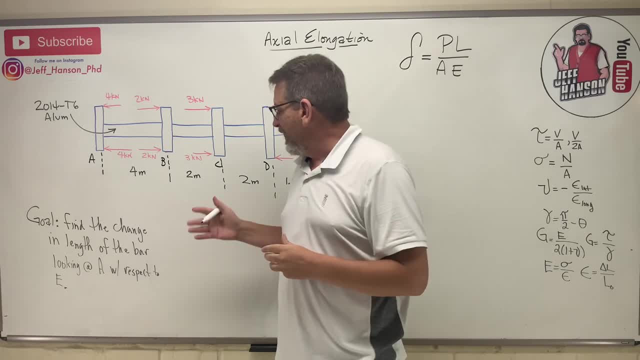 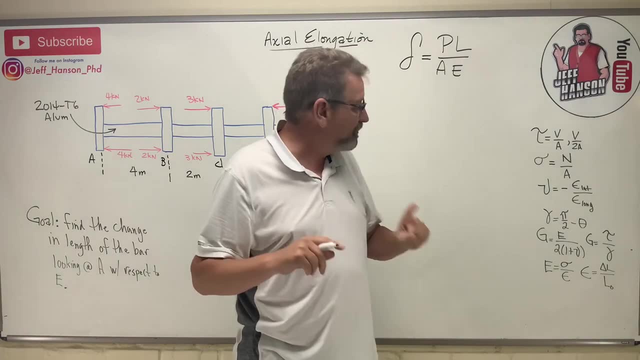 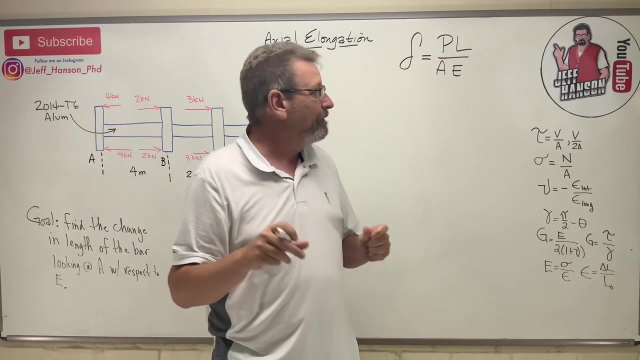 L is the length, right. so however long each segment is and we have different lengths on these segments, right, because we know about strain. remember strain, we're strained, there's strain. remember that was in changes of length per unit length. so the more of something I have when it's loaded, the 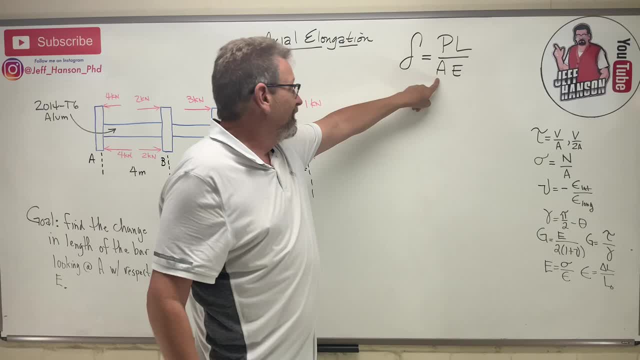 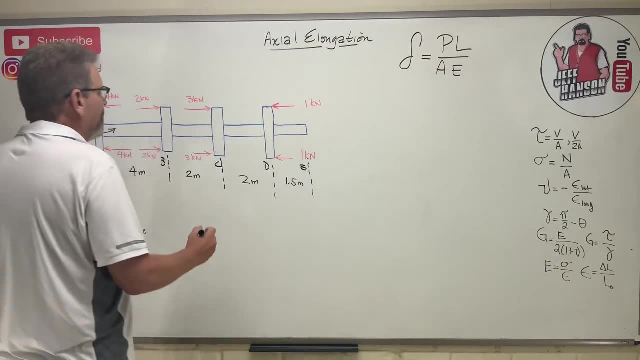 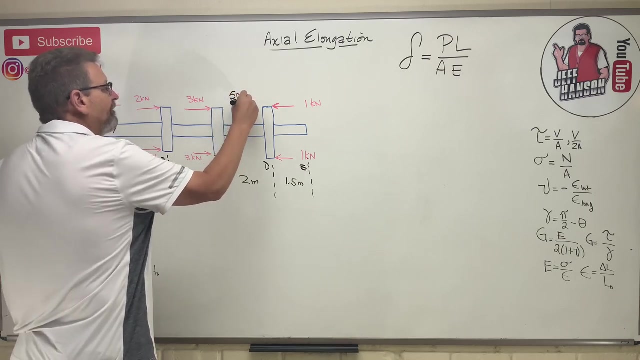 more it's going to stretch. so link definitely important. the a is just the cross-sectional area, okay, and so for this, this guy here, what we have is a 50 millimeter diameter and we got to be careful that we don't have, because all these are in meters and that's in. 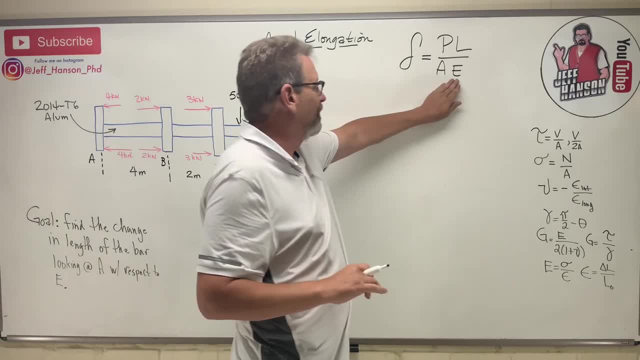 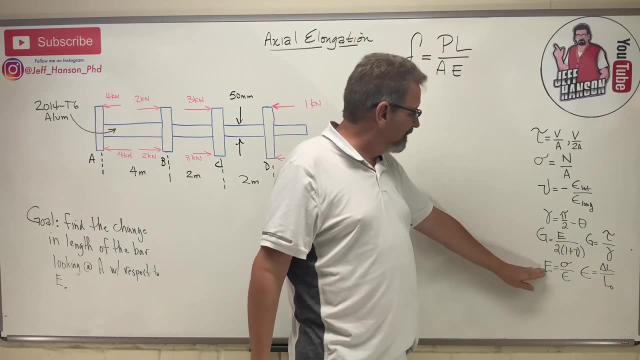 millimeters. we've got to be careful about mixed units, right. and then, of course, E. what's E? the module modulus of elasticity, and we know about how to find that, don't we? Young's modulus, uh, Hook's law, right? uh, it's rise over. run on our stress strain diagram. 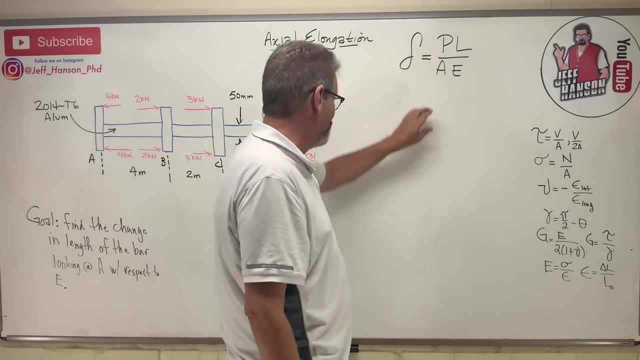 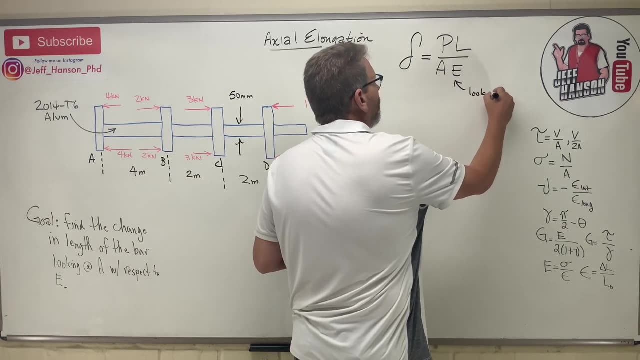 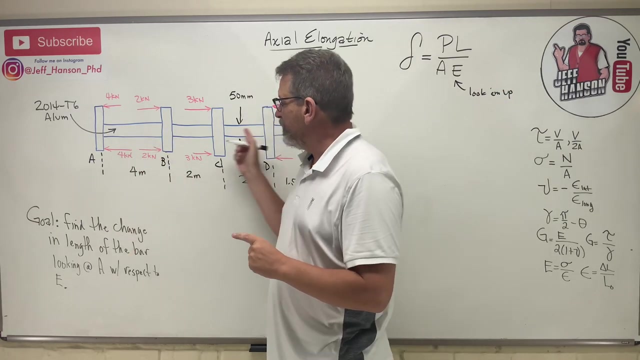 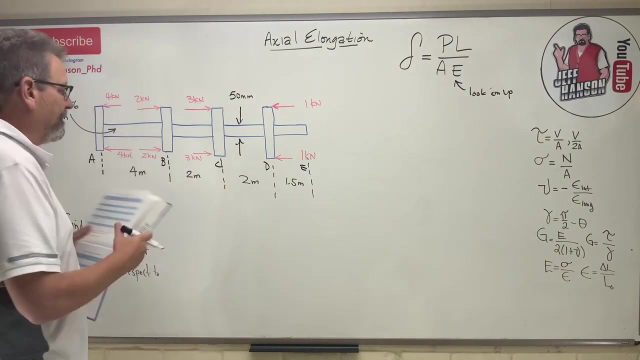 it's stress over strain, okay. and for E, this is also: uh, look them up, okay. which means if we have our book, we can just look that value up. if we know what kind of material this is- and we do- it's 2014-T6 aluminum- okay, so we get our table. we. 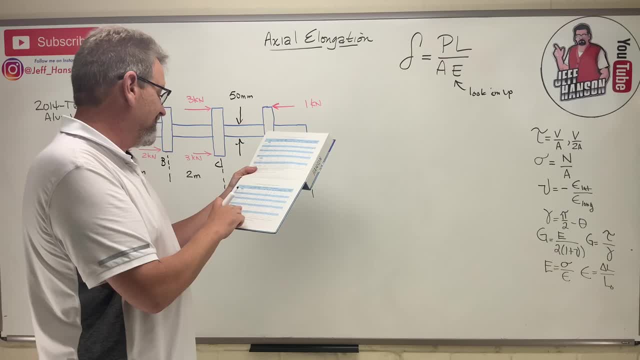 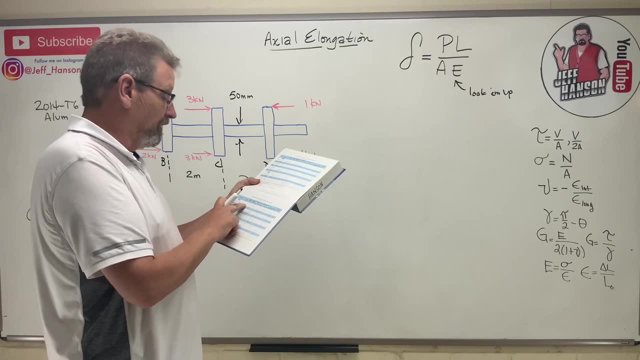 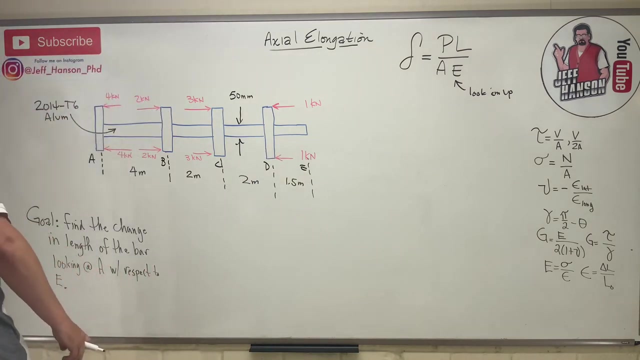 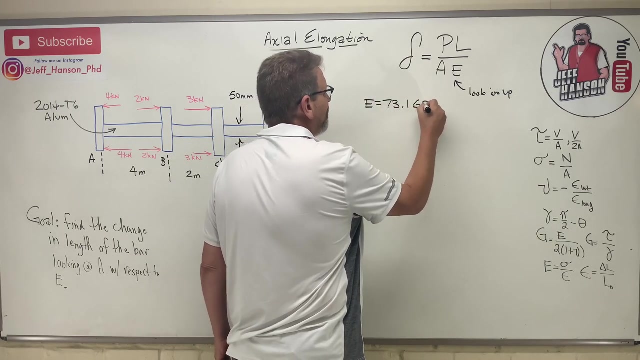 got to go to the metric table, so we go to the SI table for 2014. aluminum: hey, that's the very first one on the table and we need we need to look up E, the module elasticity, and it's 73.1 gigapascals. okay, so E equals 73.1 gigapascals, or or we can say 73 100. 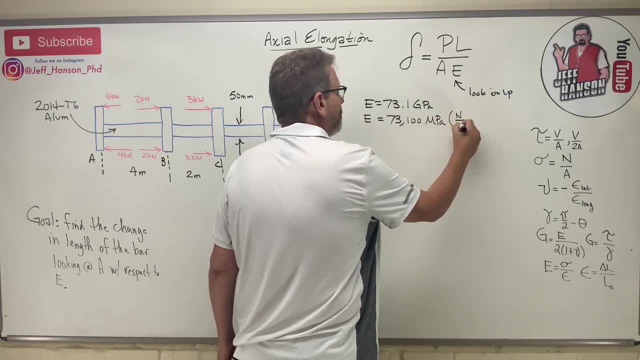 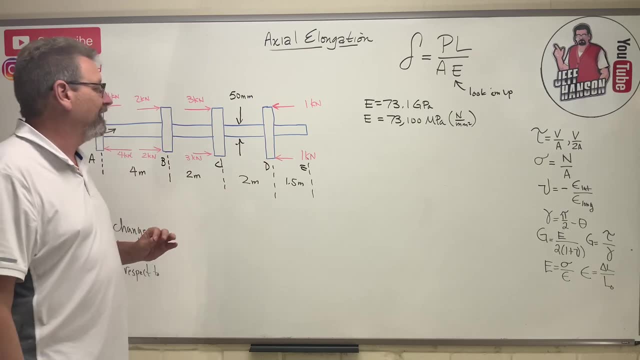 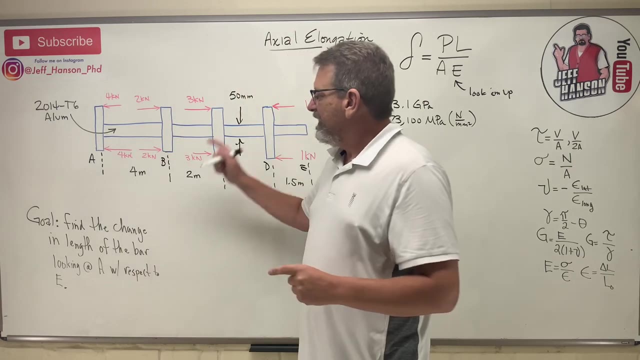 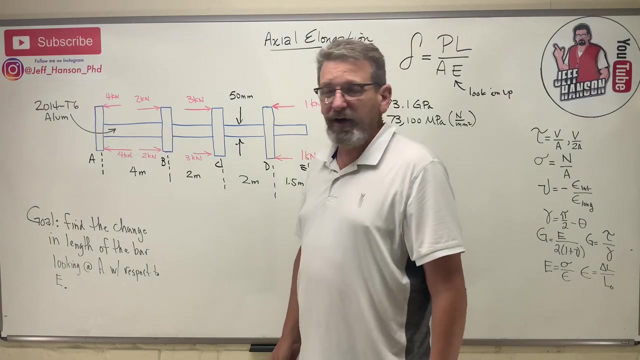 megapascals, which we know is a Newton over kilometers, squared right. if I have everything in the exact same units, it's easier for me to just cancel things out, right, okay? I think the next thing that we should do is: can you identify how much force is in each section of this shaft, okay? well, here I'm going to show you a little. 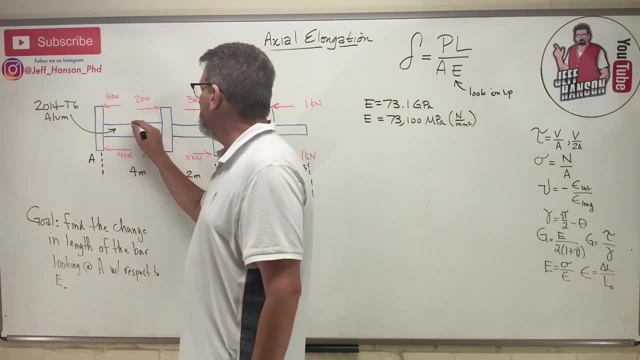 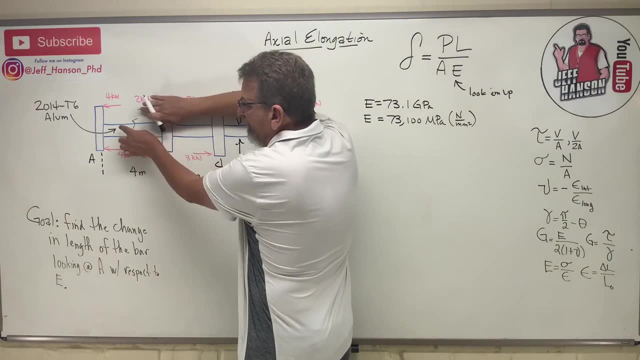 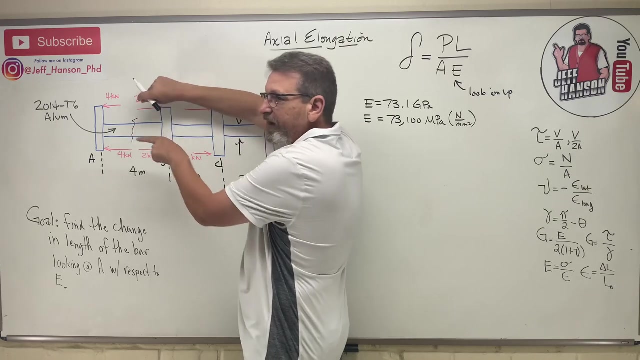 trick. here's the easiest way to do. think about if I was to cut that shaft in half right there and I was to look inside of it. okay, let's ignore everything over here, right? so what is in that shaft over there? eight kilonewtons going that way, right, four and four, eight going that way. so this section of the 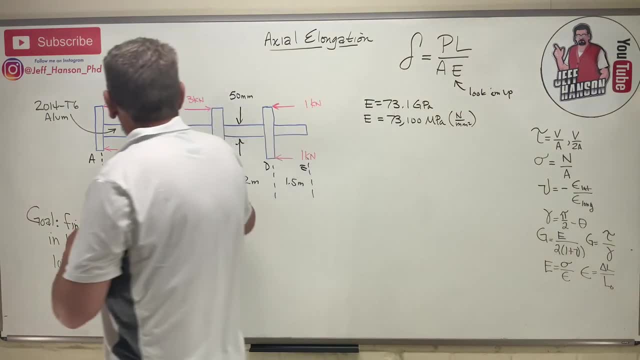 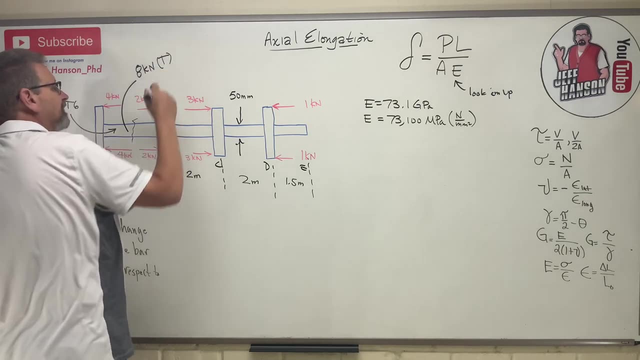 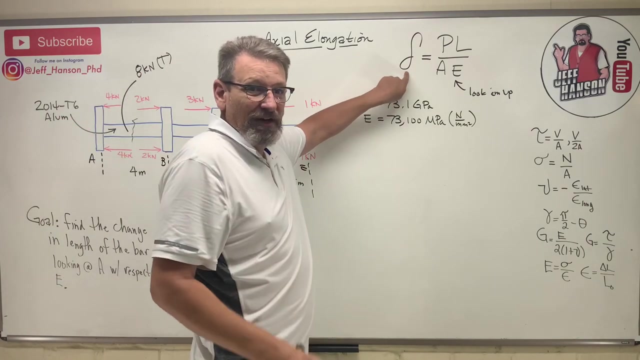 shaft is in tension, isn't it? it's in tension. so this section here has eight kilonewtons uh, tension and that's. and then, and identifying if it's in tension or compression is important, because what longer? if it's in compression, the Delta is going to be getting shorter, and so what we're going to do, 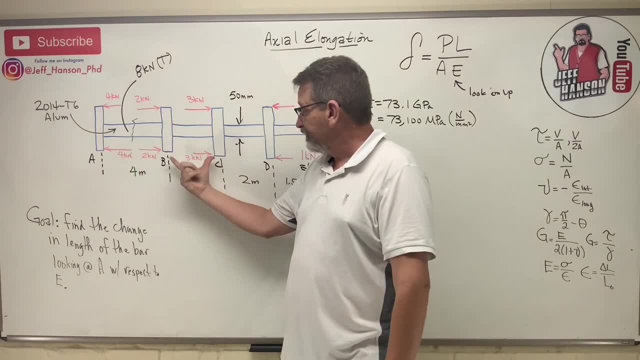 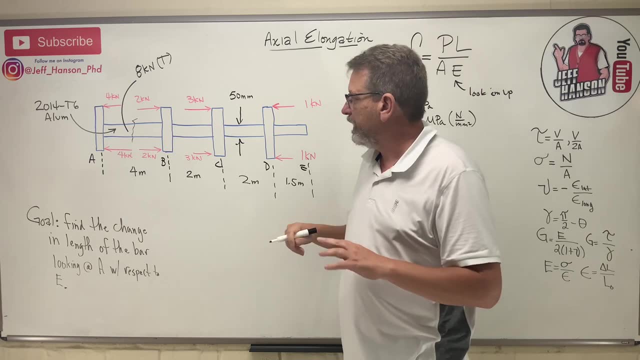 here is: we're going to add up the stretch in that section plus the stretch in that section, plus the stretch in that section, plus this last one, and that'll give us our total stretch, won't it okay? what about? oh wait a minute, that's an eight kilonewtons tension. well, what if? what if you? 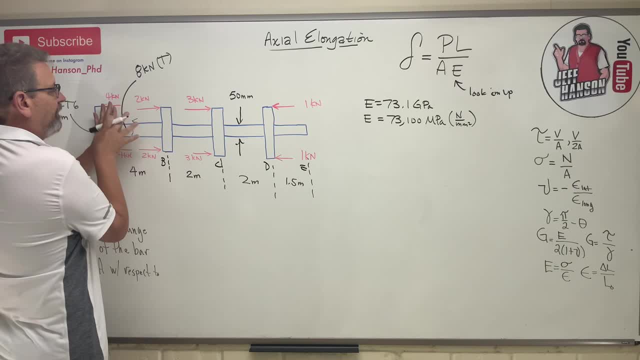 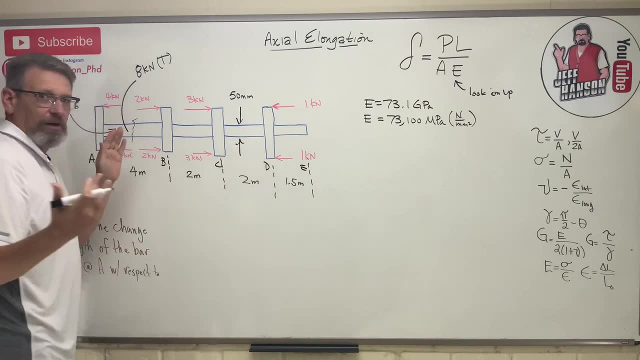 covered up this side. what do you have? okay, let's see, I got four. no, that's yeah. four plus six more than oh minus two. it's still eight kilonewtons in tension. so either side you look at, you're going to get the right answer. okay, so here, what about this section? let's cover this all up, right. 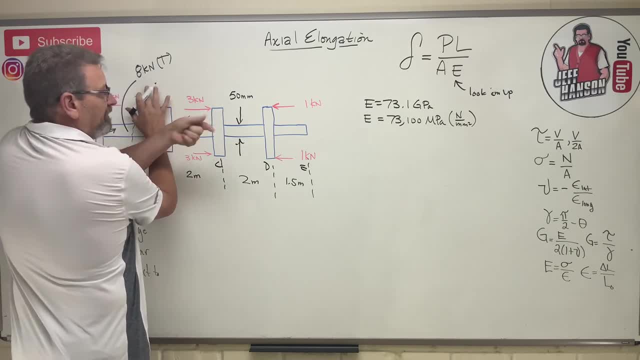 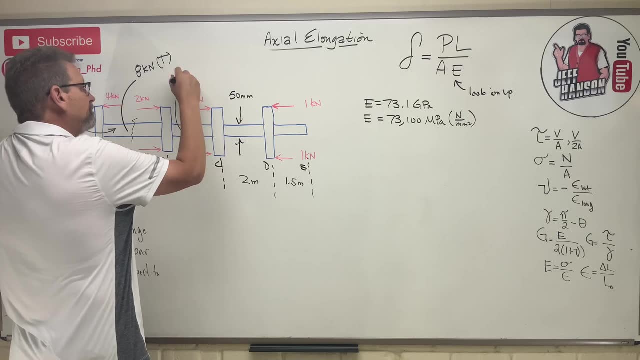 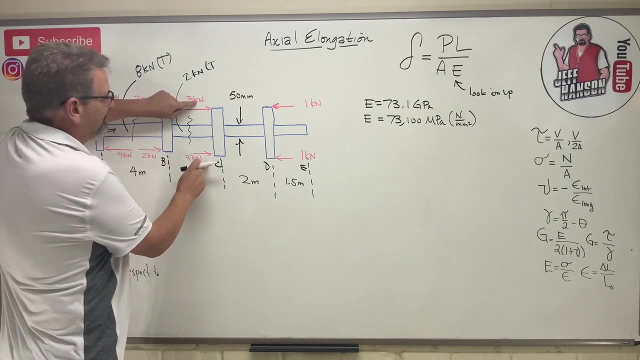 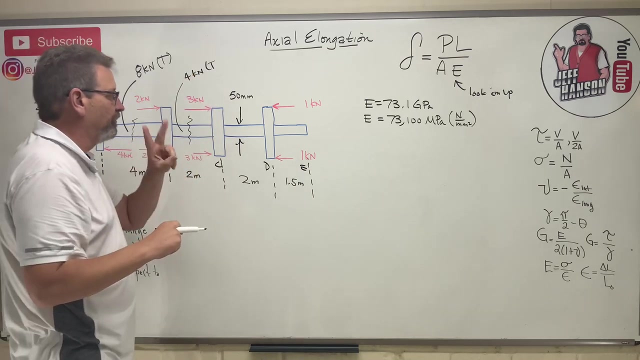 what do we have? I have three in tension and one in compression, so this one's bigger, so he's going to win, and so this winds up being two kilonewtons in tension, right? no, what are you doing? six minus two is four is four, isn't it? I forgot about? I just did one. I didn't do two of them, did I? 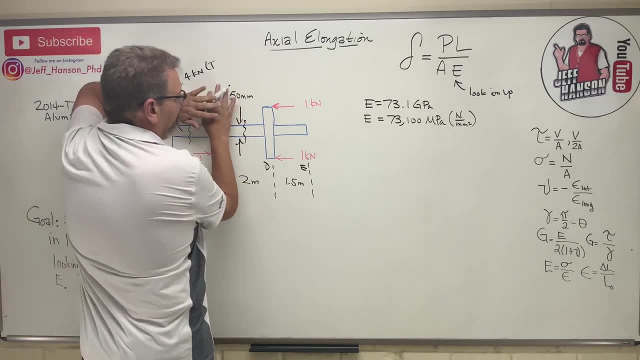 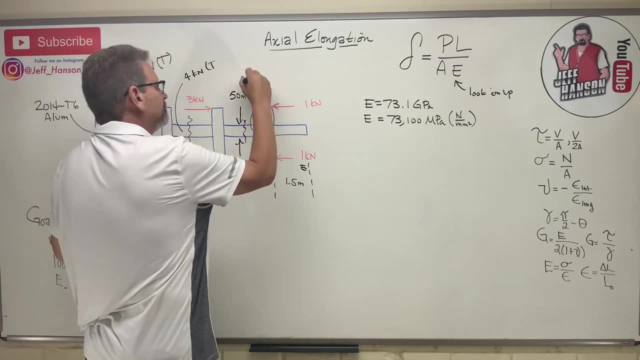 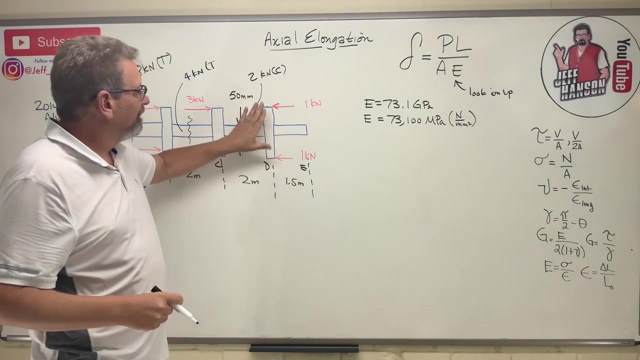 and this last section. what's going on? this last section? well, this section is actually in compression, isn't it right? it's two kilonewtons in compression, okay, and what about this guy? what do you think about this? well, if I cover everything up, right, how much is in that guy? uh? 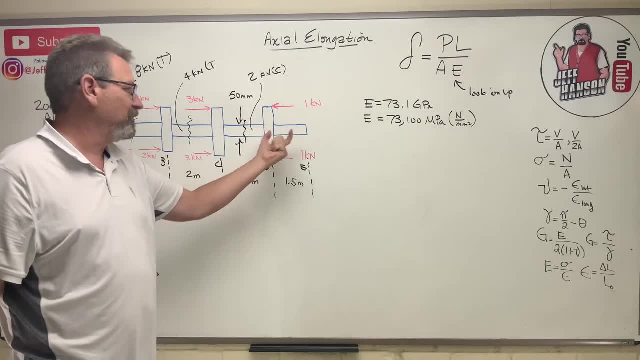 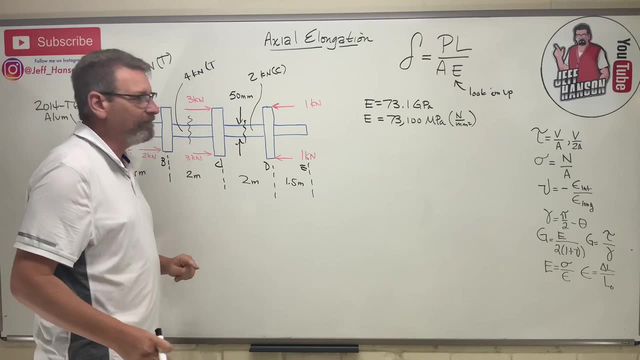 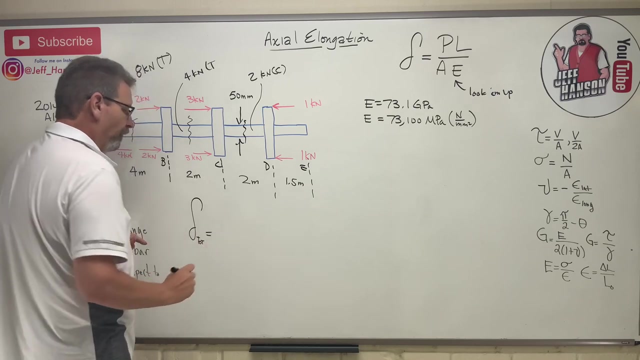 nothing. this guy is just kind of along for the ride out here, so he makes no difference. so the total elongation is going to come from this one, this one and this one. okay, so let's go, here, we go, we'll go. so Delta total is equal to all. right, I'm going to do this one. 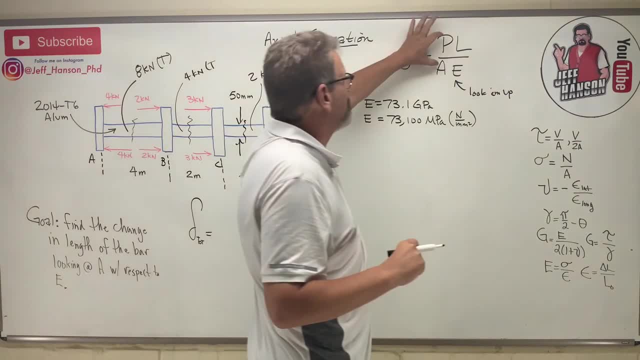 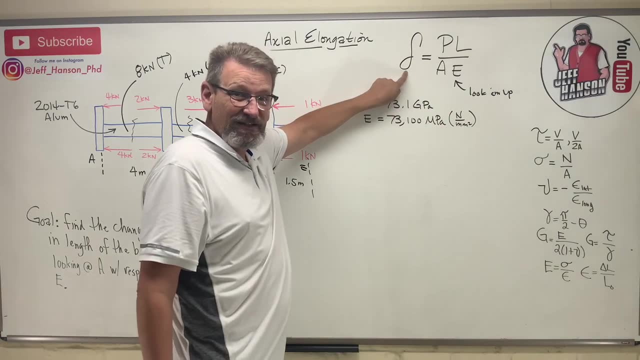 first, and I'm going to be really careful, right, when you get these big equations with a whole lot of variables in them. you got to be really careful with units, okay, because Delta is in what it's: a distance? right, it's a change in length, so it should be. let's make it in millimeters, shall we? so it's. 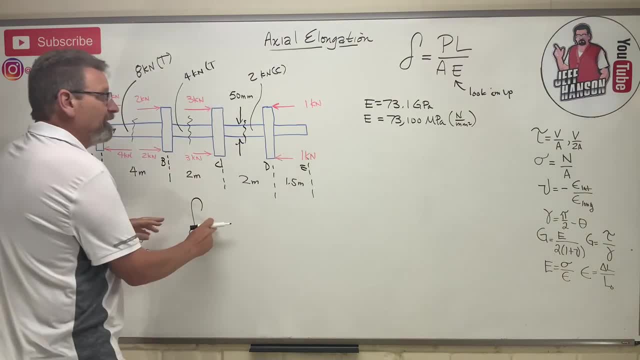 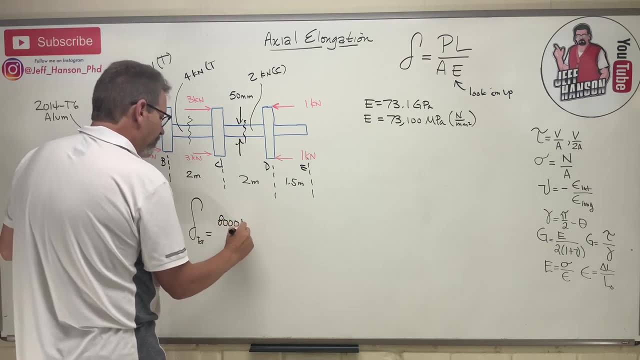 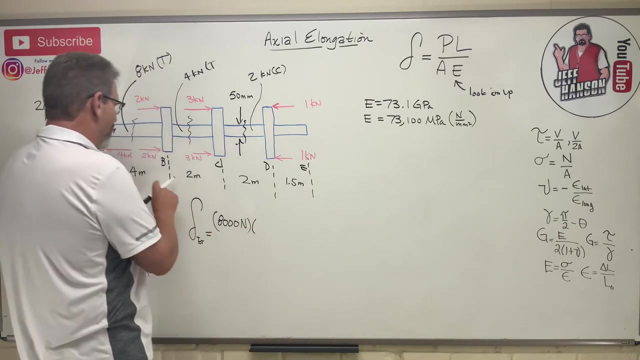 going to give us an answer in millimeters, okay, so here we go. P for this section: eight kilonewtons. I'm going to make it 8 000 Newtons. okay, it was Killa I. I made it into a 8 000. okay, times L. L is. 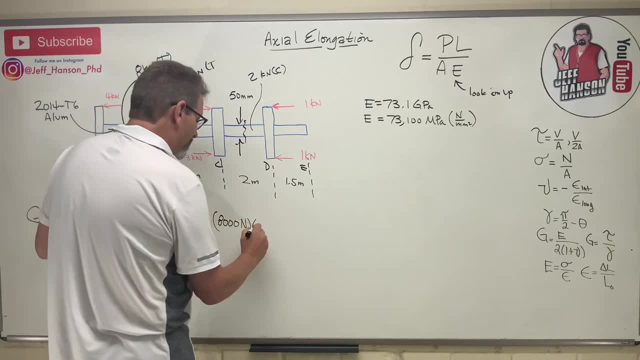 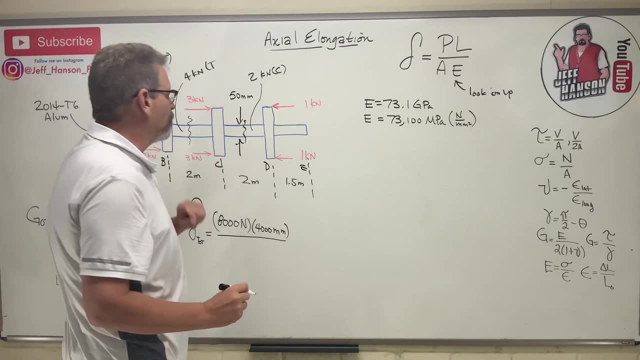 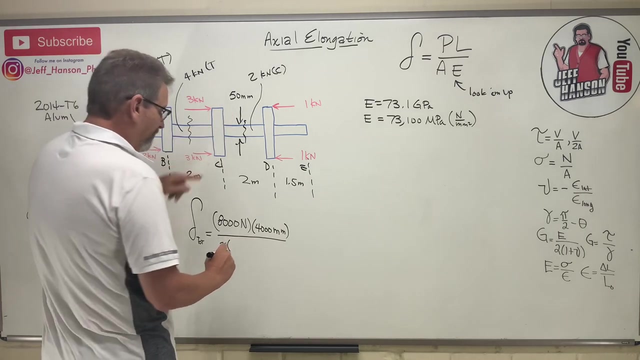 in four meters, but I'm I want everything in millimeters, so I'm going to make it four thousand millimeters, okay, divided by a: the cross-sectional area. well, that's just a pi R squared pi times. uh, the diameter is 50, so I'm going to use 25 here. okay, and that's millimeters squared, okay. 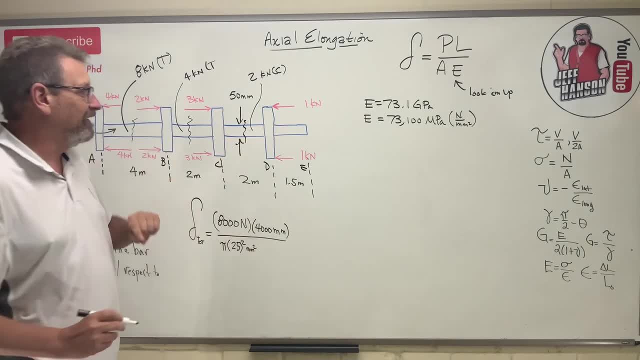 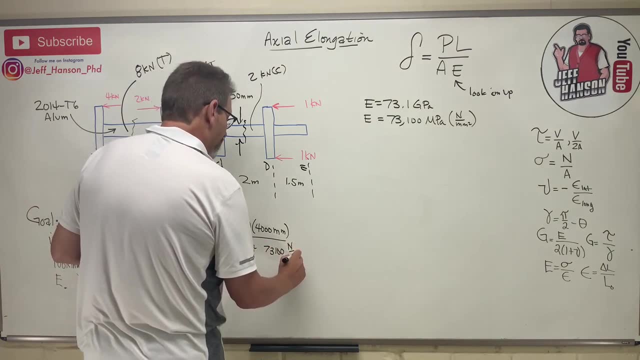 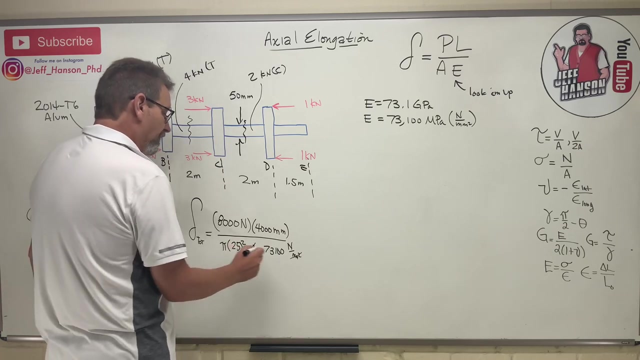 and one more thing, and I have E, and E is in. I'm going to use that. megapascals down there: 73, 100 Newtons over millimeters squared, okay, so let's see what cancels out here. millimeter squared cancels out. um, there's a Newton, there's a Newton, and I'm left with just millimeters. that's what I want, okay. 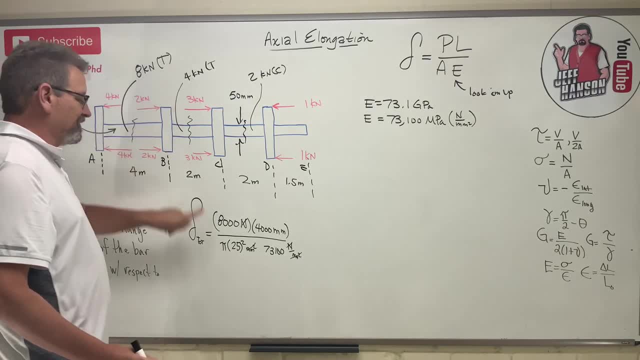 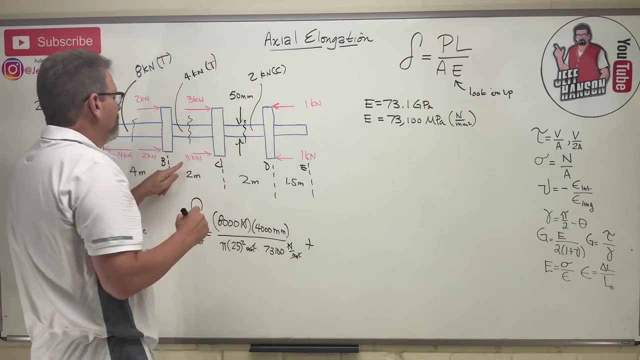 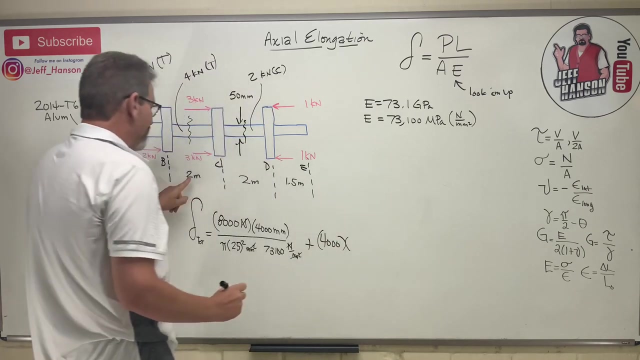 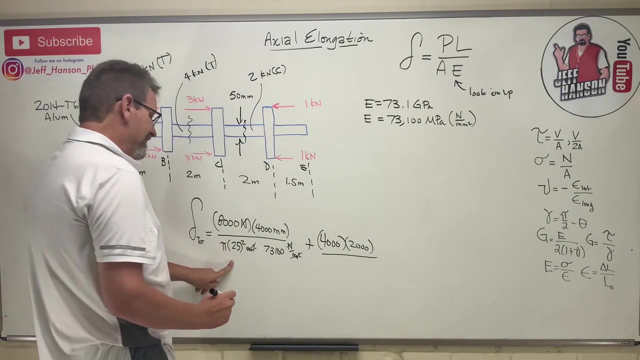 and this section here is going to be stretching since it's in tension. so he's positive. next section, also positive, stretching right, tension, tension, um, and it's going to be four thousand times the length of that guy, two thousand divided by same exact thing, isn't it? 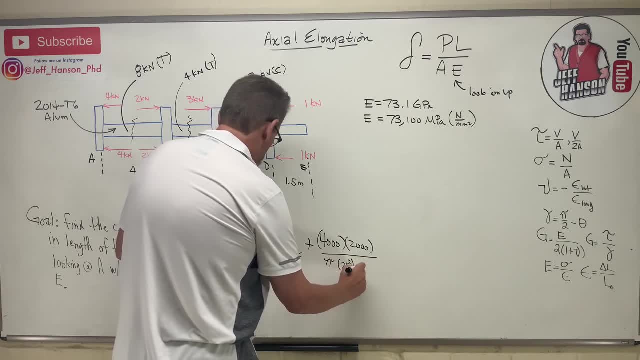 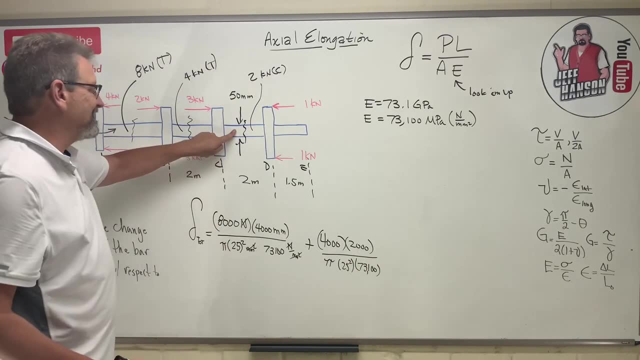 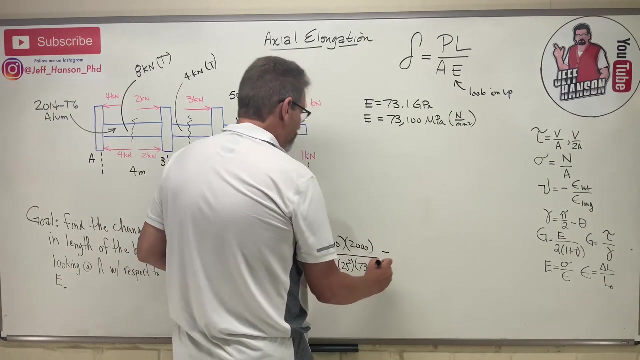 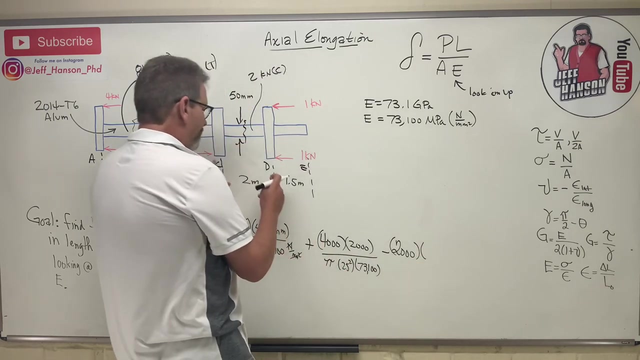 pi times 25, squared times 73, 100, okay. and then finally this last section here and it's in compression, so that section is going to be shrinking, so I'm going to make him negative. right extension times 2000: okay. times the length: 2000. 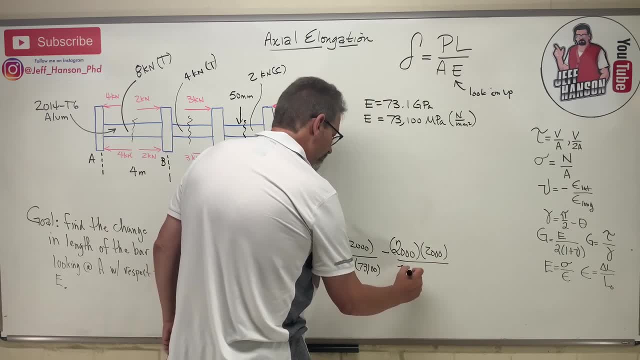 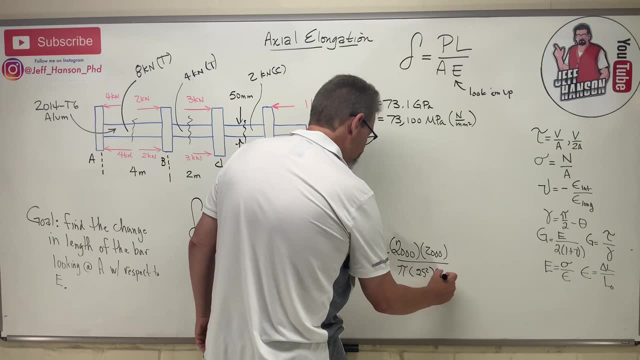 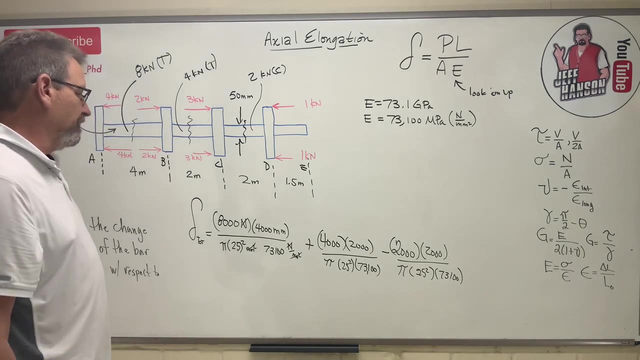 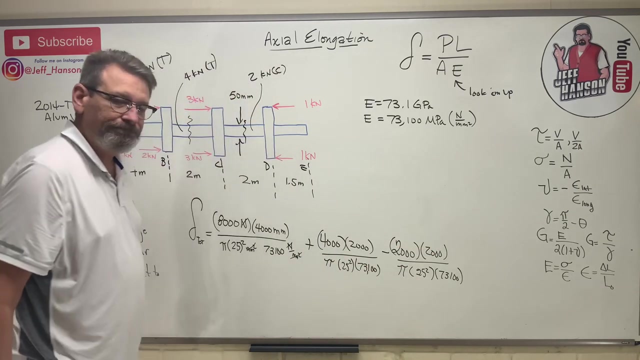 divided by pipad times 25, squared times 73, 100 vois, no in-on-tab, all the way he said so tremendous of all of these. add the tops, all of those together, the, the numerators, and then it's like I'm factored out all of those denominators, and I'll do that at. 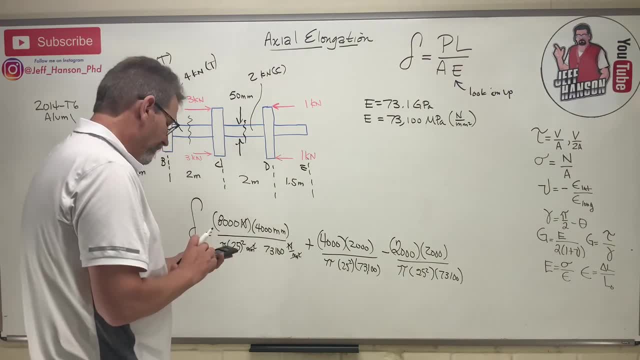 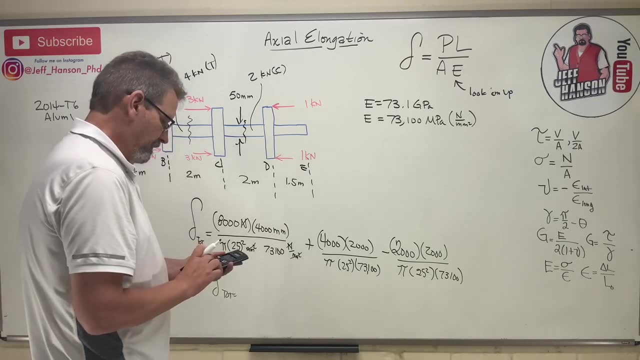 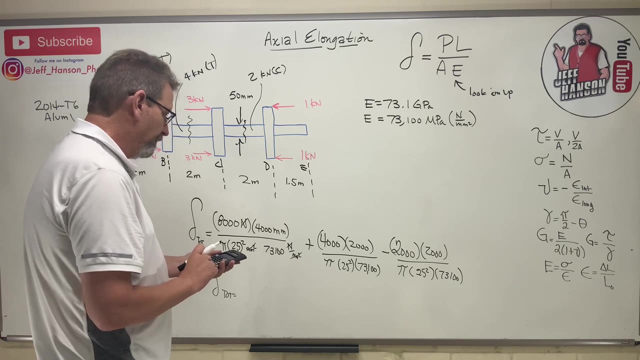 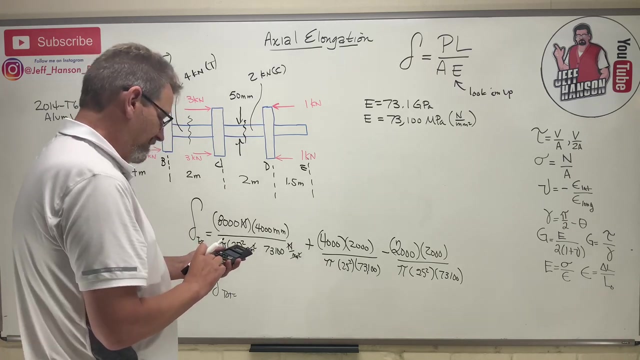 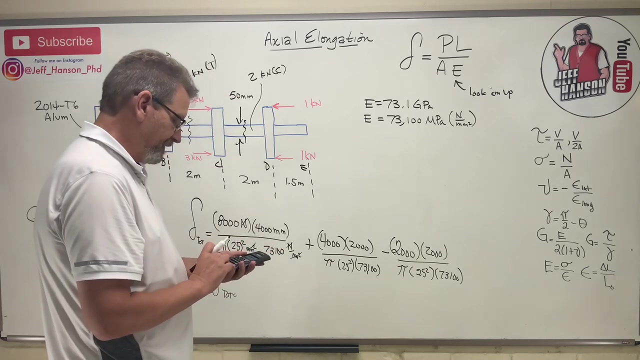 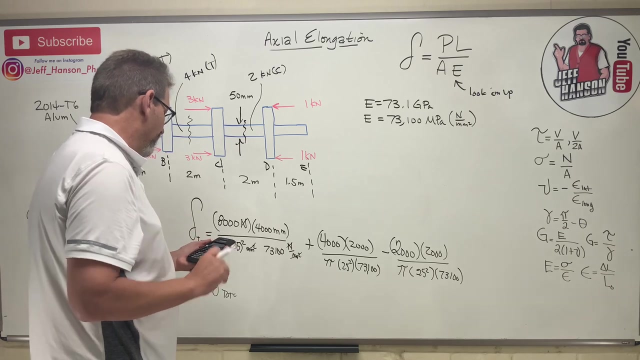 the end is that cool, that's cool, okay, here we go. so Delta total is equal to clear, 8,000 times 4,000, plus 4,000 times 2,000, minus 2,000 times 2- right, no times 2,000 equals, all right, a big number. and then that number I'm gonna divide by: 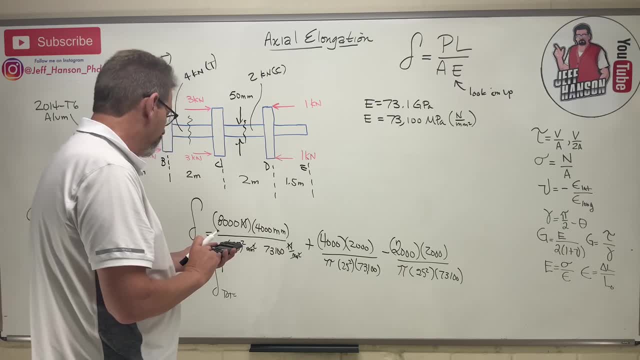 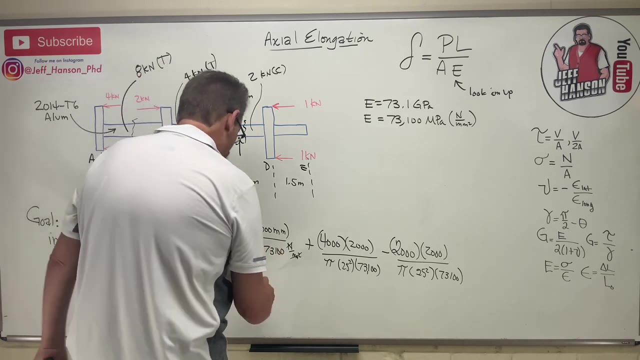 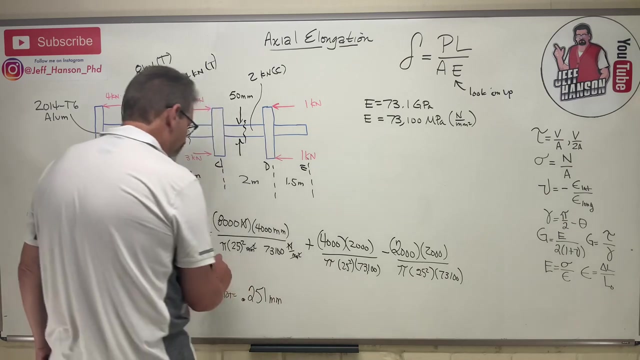 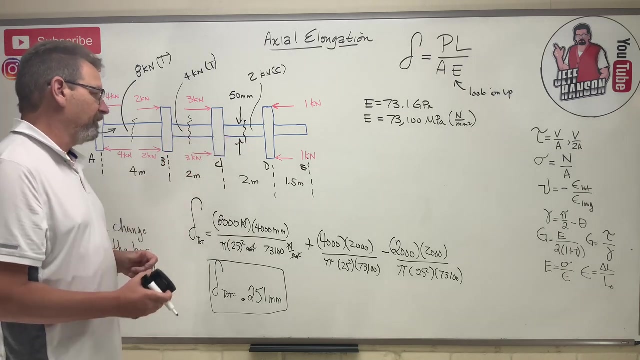 divided by PI equals, divided by 25 squared equals and then divided by 73,100 equals, okay, 0.2508, okay, so the whole thing right. this one stretched, that one's stretched, stretched that one's stretched and that would compressed. could I find the stretch in each one of those? yeah, I.